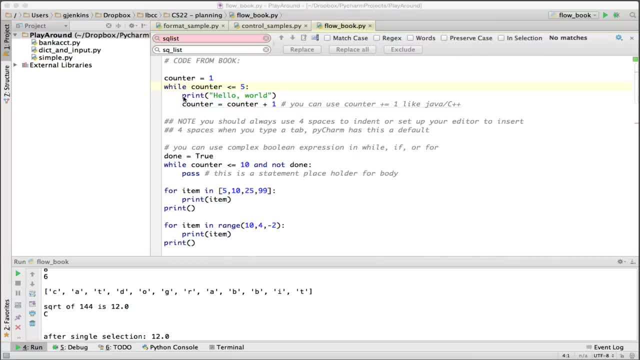 the colon and the indent. So everything indented at this level will be the body of the while loop And as soon as you go back to the previous indent level, it knows that's not part of the loop. So this loop will count from one until the counter is five and print hello And it will increment the 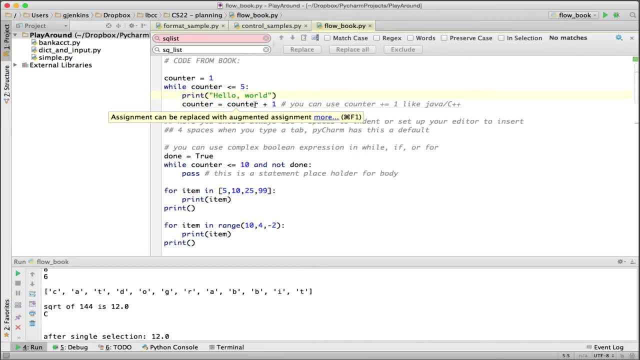 counter inside of the loop And it will increment the counter inside of the loop And it will print the counter inside. I'm also pointing out here, and I don't think the book does it, but you could replace this statement here with this: counter plus equals one. 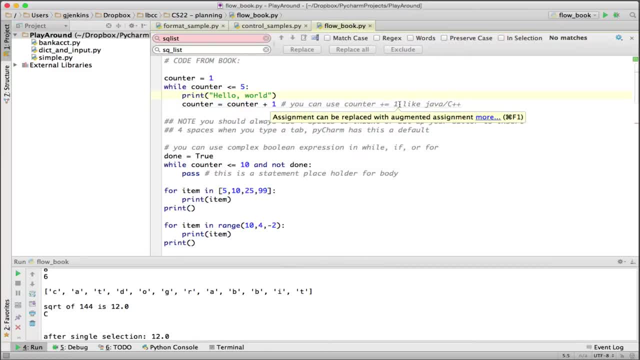 And you may remember that from your C++ or Java class is a statement to do, a shortcut for adding something to counter. Python doesn't have the plus plus operator like in C++ and Java. Here's another example they have in the book. You can have a while and then you can have a. 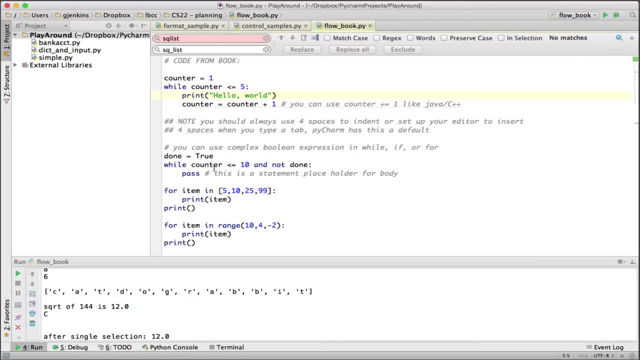 boolean expression that's more complex. So here they have two terms that result true and false. One of them is a flag And they use the word not in front of it And they use the and operator. So they're combining two true or false results with an and, And they'll keep doing the loop until 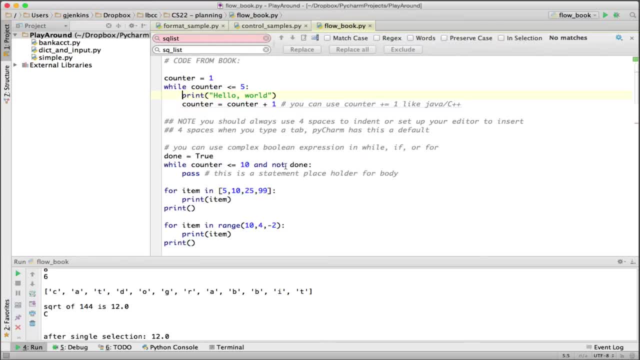 either this is true or while this is true and this one is not true. So I set done to true here. it will properly exit because the counter never changes. I use a pass statement, so this loop actually will stop because done is set to true initially. 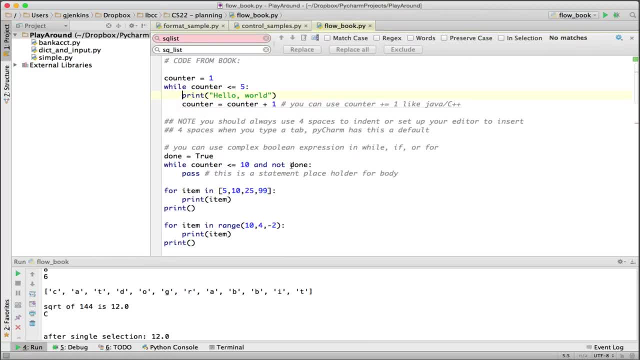 so it says and not done. this will become false and that will cause the loop to not execute. I also have placed a pass statement. This is a special statement. you can put anywhere you have a body of a compound statement or even a body of a method. 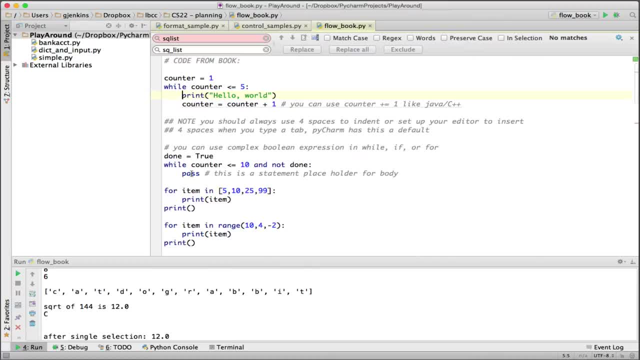 and it's basically a placeholder for the body that says do nothing. If you try to do a loop and you leave out all the statements after the loop, it will be a syntax error. The next example is a for loop, So the for loop always works by. 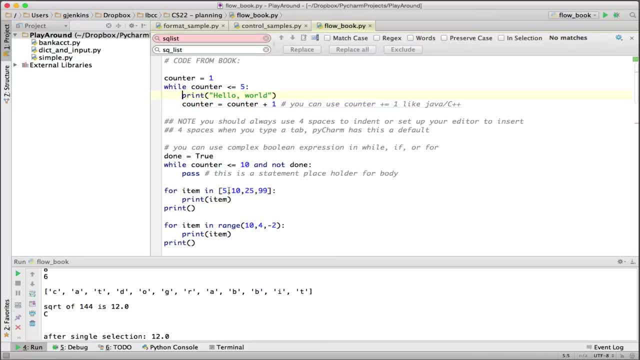 for some item in something that iterates through a list of things. So item will assume each object that's in the list of things and the body of the loop. so again we have the colon, the mark that we're about to start the body. 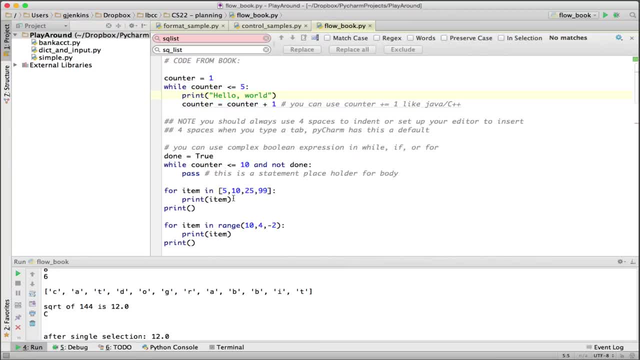 we end it in. so the body in this one consists of one statement, so it's going to. item will be: first it will be five, it's going to print five, and then it's going to be ten. it's going to print ten. 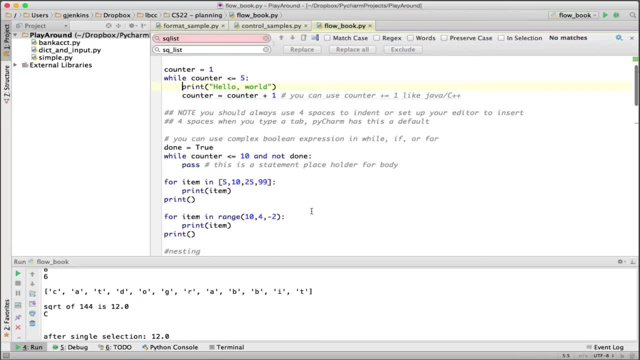 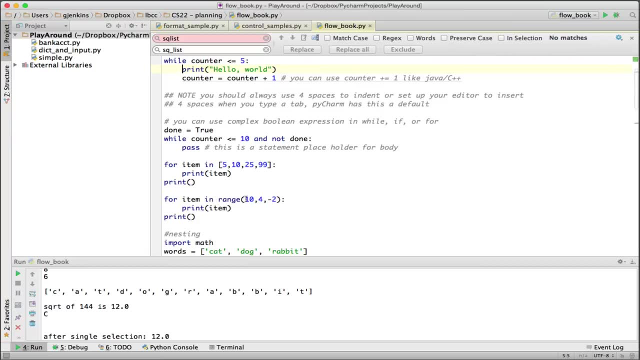 and so on. it will print these values. You can also use range. you can use anything on the right side of the end. it creates a sequence of values. So range creates a sequence of values. In fact, technically that uh. 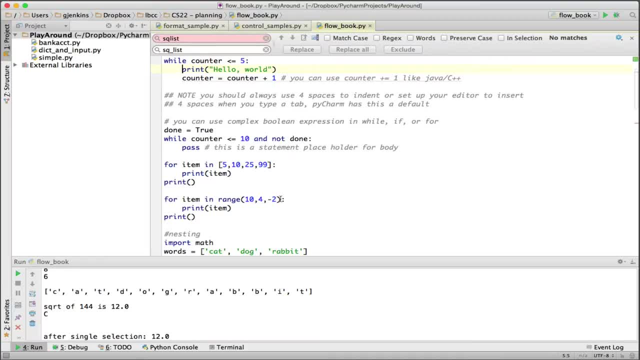 the thing on the right is what's called an iterator. It iterates through a range of values And so it's going to print out ten to four going minus two. so it's going to count down two at a time and uhit actually. 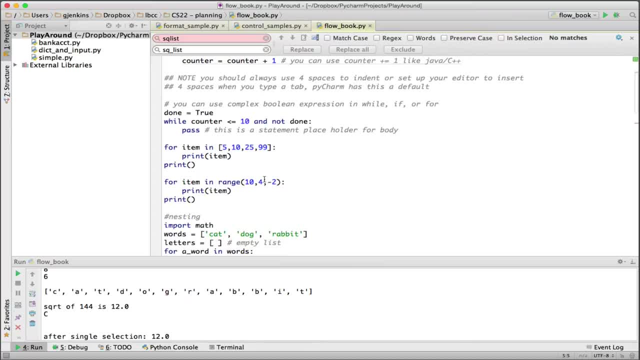 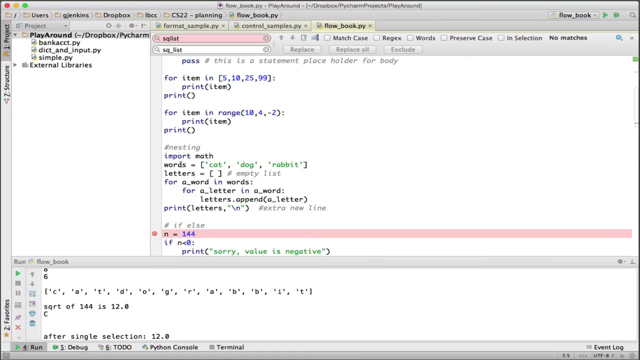 will stop before four. Remember 4 is always the inner range. The second number is always just past where it stops. You can also nest structures. So here's a more complex example. We import math. We're going to use that later module math. 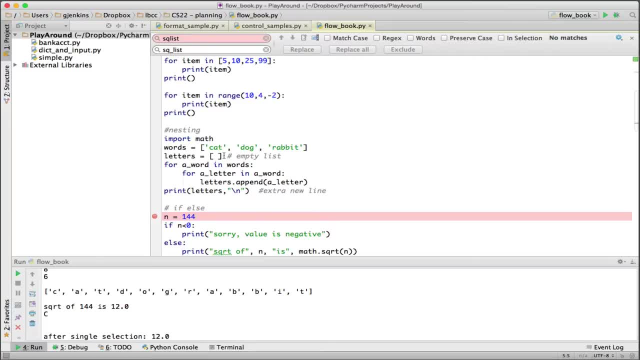 It sets a list of words And it makes an empty list. we're going to fill in which is empty And then the outer loop will loop through each word. So a word will be cat the first time through the loop And then it will be dog through this loop. 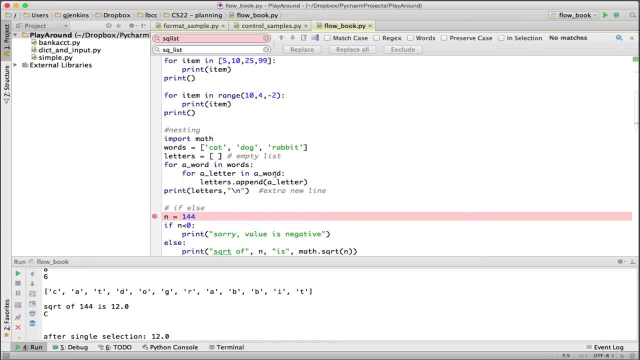 And then it will be rabbit. The inner loop will then work on that word and have a loop through each letter of the string that it got here. So it will loop through C A T in the inner loop And when it's all done with C A T it goes back to the outer. 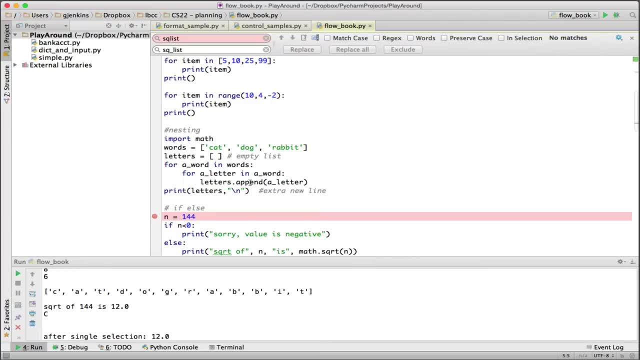 loop and gets the next word, And what the inner loop does is just append each letter to letters. So what it does, you give this a list of words And it's going to basically string all letters out individually as items And you'll see when it prints it. it's a list. 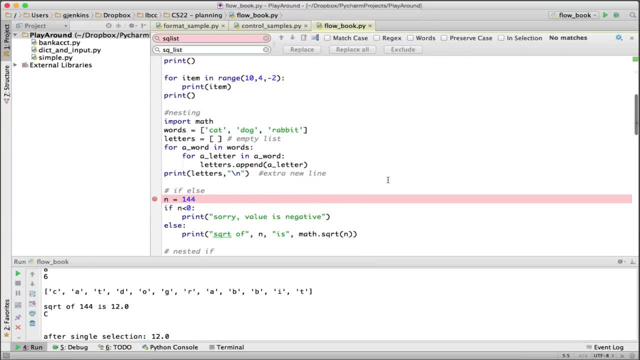 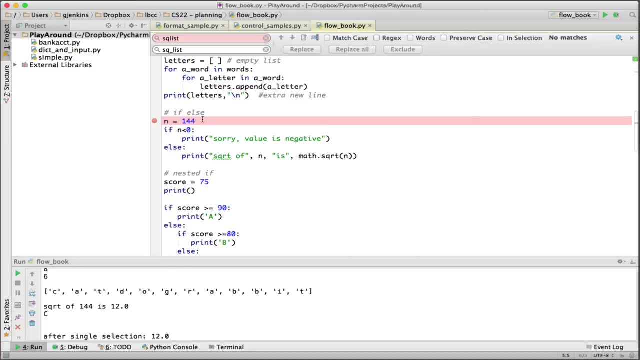 of individual letters that are all these words. Here's an if-else, So it's also what you might expect from everything we covered so far. You say: if you have a Boolean expression, a colon, You have a body which can be. 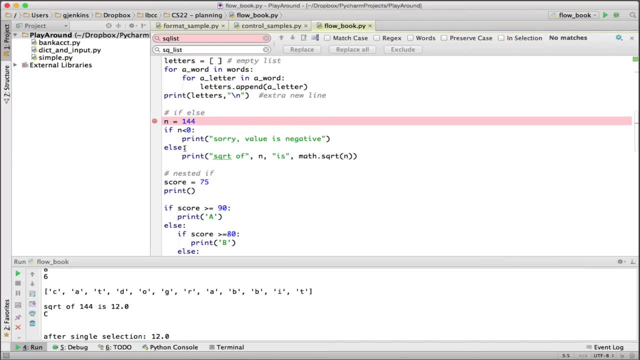 One or more statements. Then you go back out to your previous intent level and have an else with a colon, And then you have the body of the else, which can be one or more statements. Now here's a nested if statement. This is typically very messy to do because you have to. 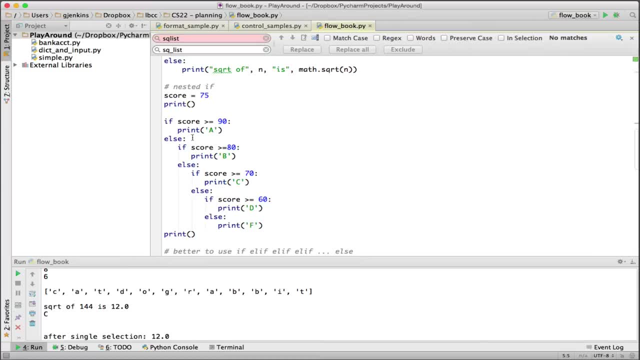 You have if and you have what happens if it's if, And then you have else, And so this if-else is the whole Body of this else, And this if-else is the whole body of this else, and so on. So each if is nested inside of an else. 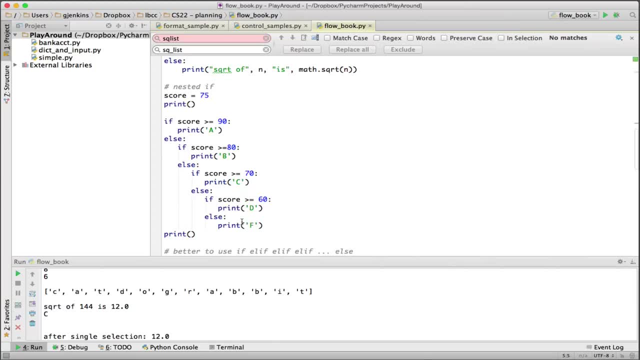 So it turns out this is a common structure to do when you have some value or something, you're comparing and you're making a multi-way decision is what we call it. You'll notice the last else is just else. And then you print f. 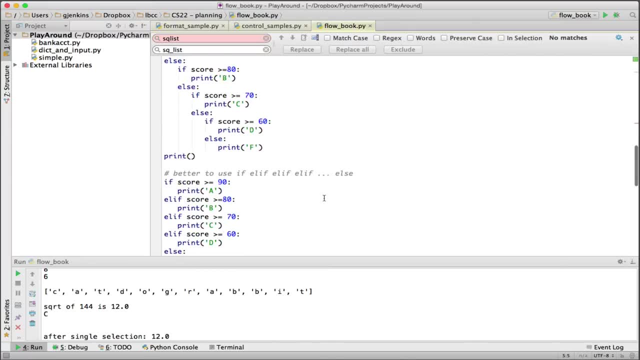 So there's another way of doing this, And that's That's what it shows here. It's called the if, l-if, l-if, l-if, else statement, So the l-if stands for else, if. So it stands for what you're doing here. 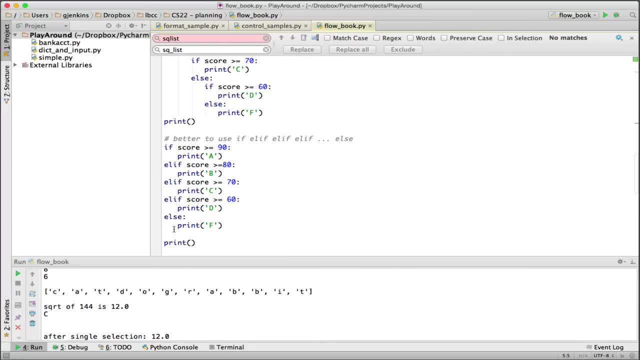 But now you can put it all in a nice, much flatter structure. There's not as much indenting And it's easier to read. You also have if with just a single branch. So if this is true, it does that. 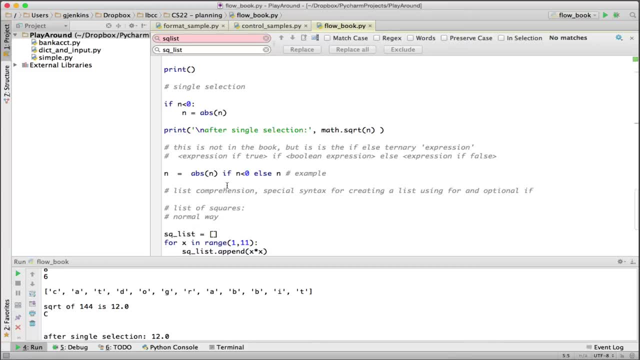 And this isn't in the book. but there's a special ternary expression. It's like the ternary operator in C++ and Java, which you probably have forgotten by now. But this is an expression, It's not a statement And the syntax is: you put some expression of true. 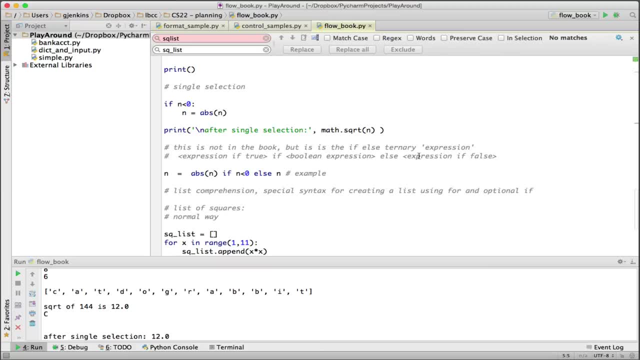 if some Boolean expression else, some expression of false, So in this case we have absolute value of n, if in, If n is negative, So we're testing. if n is negative, So if n is negative, the result of this expression: 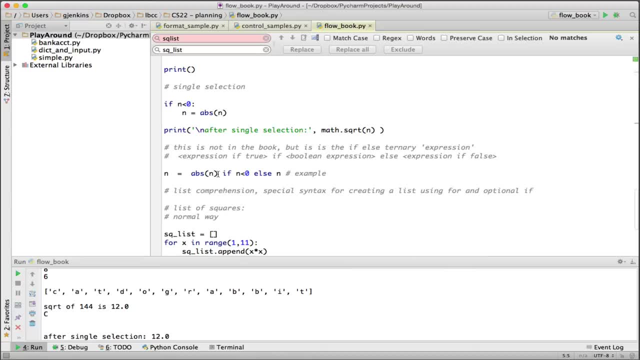 will be absolute value of n, So it's going to change it to positive If this if is false, it's just going to return n as it is. So this expression will return either the value on the far left or the far right, depending on the Boolean expression in the middle. 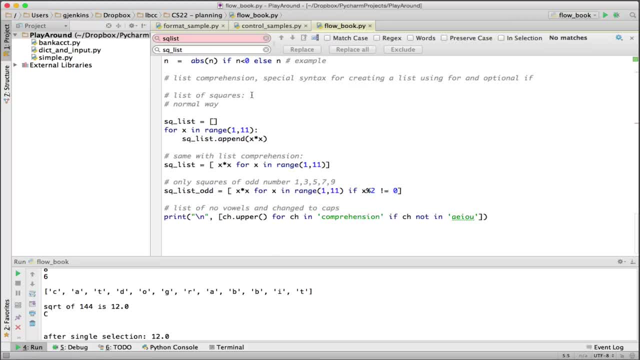 Now Let's talk about a shortcut for creating lists, because you do it so often, And they built some special way in Python to do that called list comprehension, And list comprehension allows you to use basically a loop like a for loop to create a list. 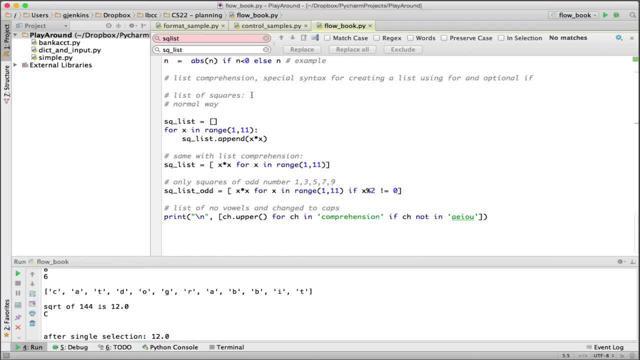 And it has an optional, if you can add, that would filter your results. So here's your normal way of creating, say, a list of just the squares of 1 through 10.. So we set up a empty list called square list. Then we say for x in range 1 to 11.. 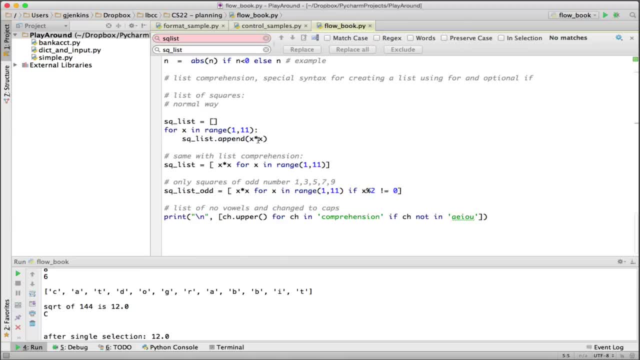 So that's going to count from 1 to 10.. And so x in here is going to be 1 to 10 as it goes through the loop. So every time the loop it's going to take 1 and multiply it by itself. 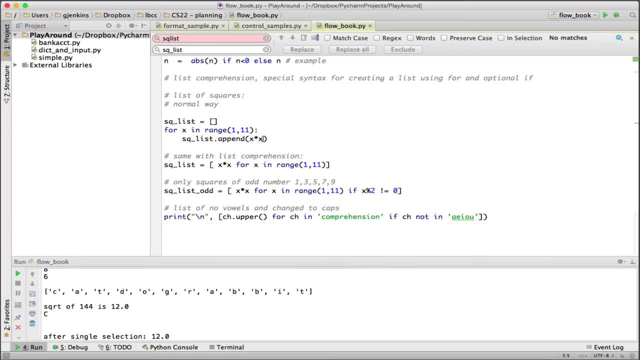 and append that to the list And it'll do 2, multiply it by itself so that'll be the square of 2.. So when this is done, you'll get the list of squares. But this is the same example as this, but using list comprehension. 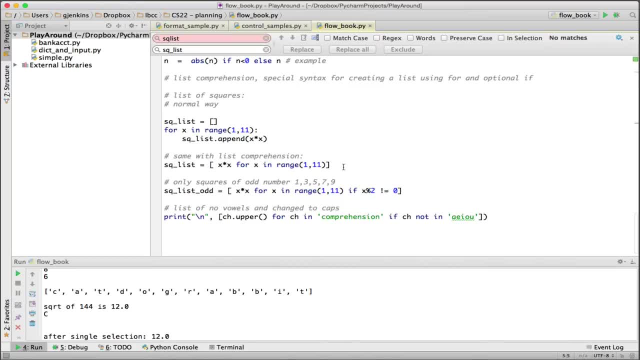 So you can see you can do it much simply And it's actually a little more readable. So it says basically: make a square list. that equals start a list. make it the square of x for x in the range 1 to 11.. 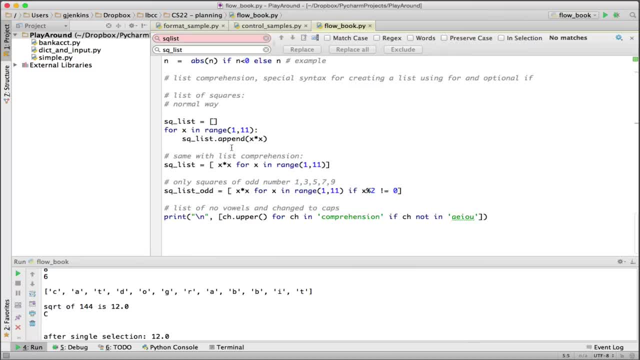 And then if you want to only do the squares of the odd numbers, you can use something like this: So you have square list: odd equals. start a list. start a list. do the square for x in range of 1 through 11,. 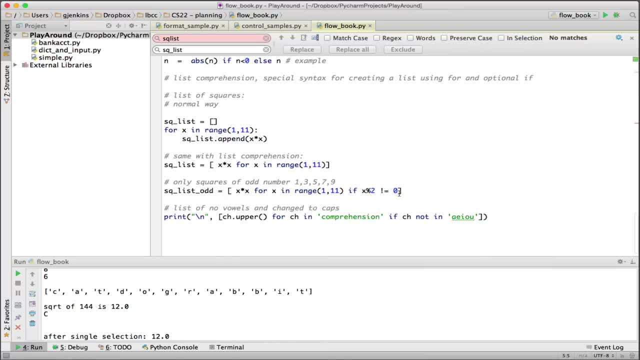 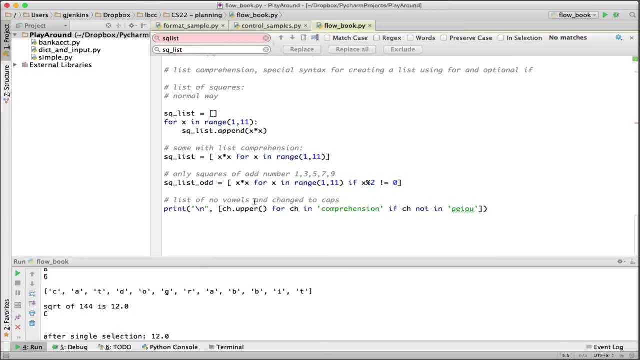 but only if x modulus 2 is not equal to 0.. This is testing. if it's odd, If this filter is not true, it doesn't add x to this list value. And then here's a special one. This is a list of no vowels.